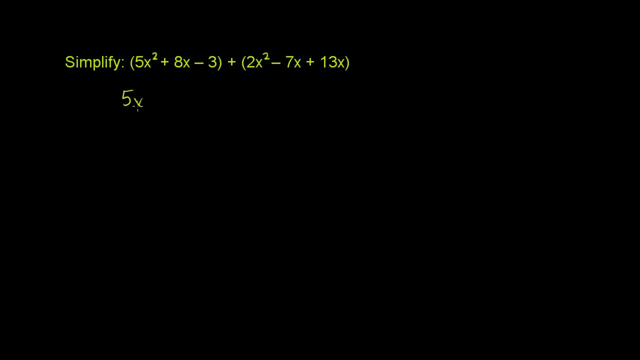 So we have 5x squared plus 8x, minus 3, plus 2x squared. If this was a minus, then we'd have to distribute the negative sign. but it's not. So: plus 2x squared, minus 7x, plus 13x. 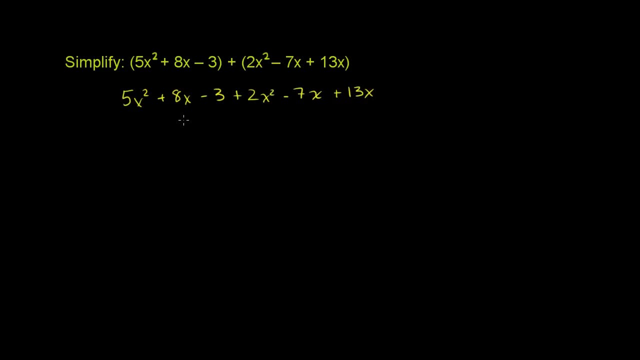 Now let's just look at the different terms that have different degrees of x. Let's start with the x squared terms. So you have a 5x squared term here And you have a 2x squared term right there. So 5 of something plus 2 of that same something is going to be 7 of that something. 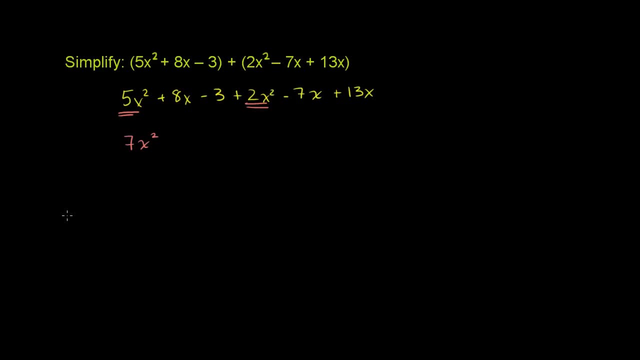 So that's going to be 7x squared. And then let's look at the x terms here. So we have an 8x right there, We have a minus 7x And then we have a plus 13x. So if you have 8 of something minus 7 of something, you're just going to have 1 of that something. 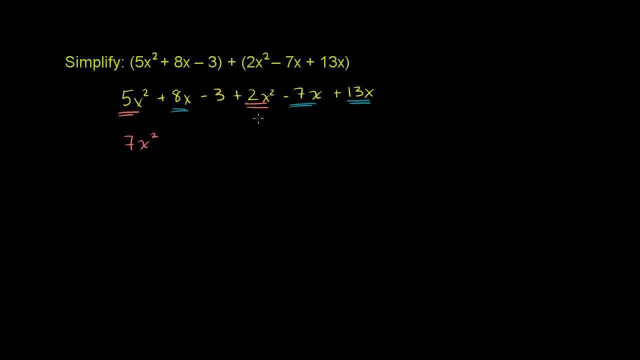 And then, if you add 14 of that, something more, you're going to have 15.. So this is going to be plus 15.. 8x minus 7x- oh sorry, you're going to have 14x. 8 minus 7 is 1, plus 13 is 14.. 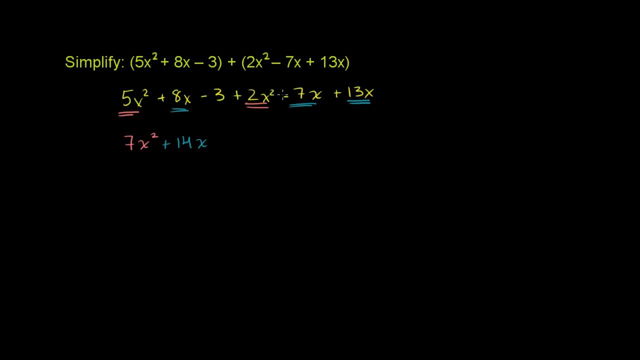 Plus 14x. That's these three terms: 8x minus 7x, plus 13x, And then, finally, you have a negative 3, or minus 3,, depending on how you want to view it, And that's the only constant term. 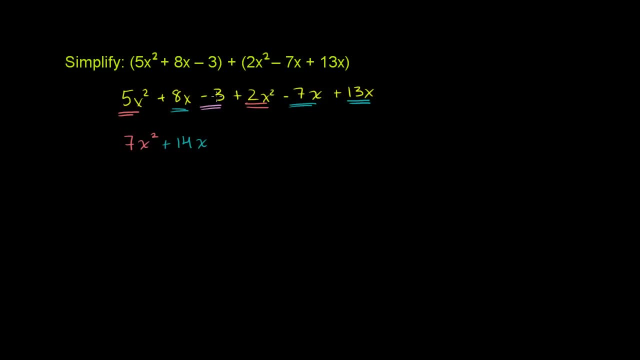 You can imagine you could say it's x times x to the 0. But it's a constant term. It's not being multiplied by x And that's the only one there. so minus 3.. And we've simplified it As far as we can go. we are done.